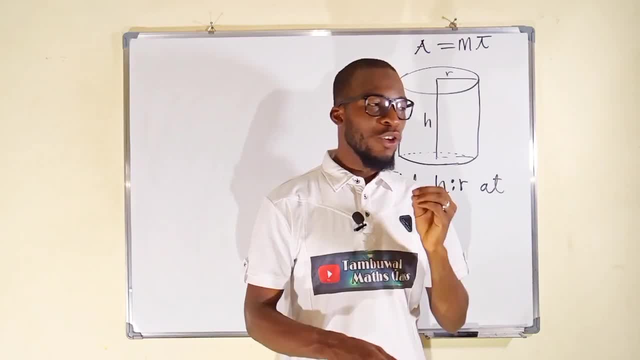 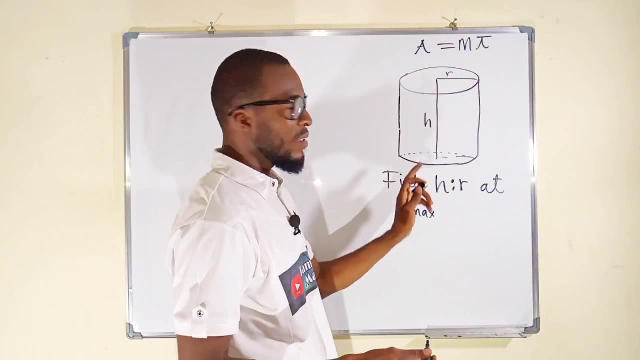 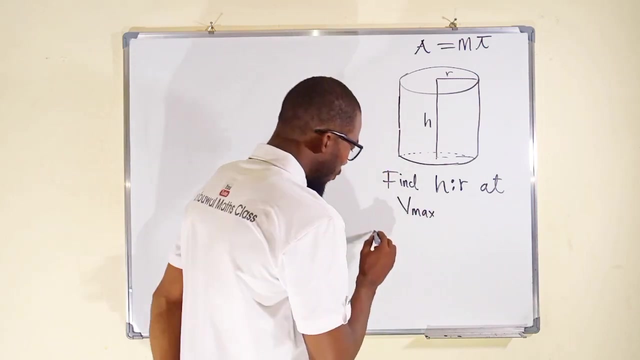 important formulas. One is for the volume and the other one is for the total surface area. For the volume, you know, it is the area of the base multiplied by the height, and the base is a cycle Area of a cycle. is pi r squared multiplied by h? is pi r squared h, So v is equal. 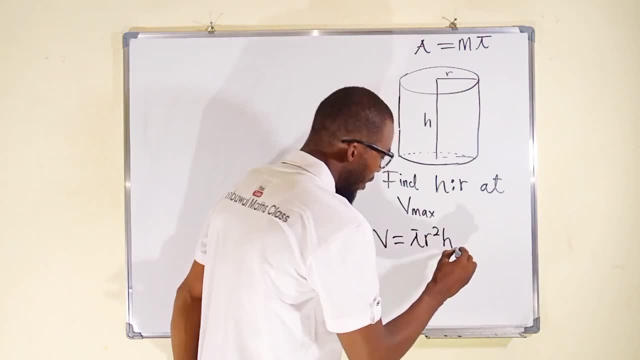 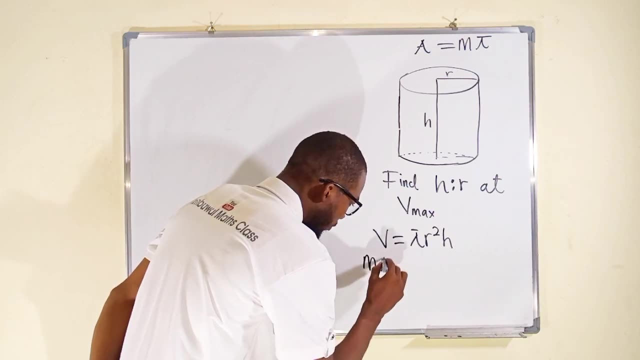 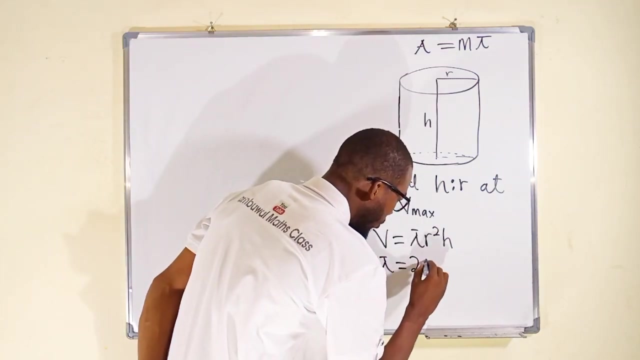 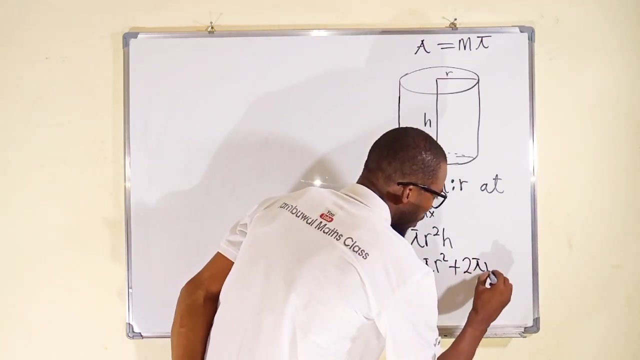 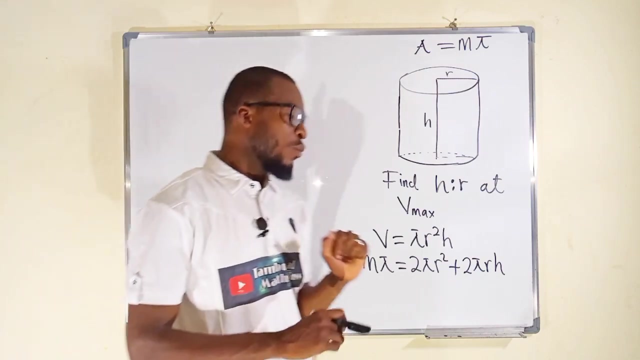 to pi r squared h. Then for the total surface area, which is given as m pi, m pi will be equal to the two cycles areas is now going to be equal to two pi r squared. Then the cop surface is two pi r h. So look at the first equation. The first equation is expressed in terms of the 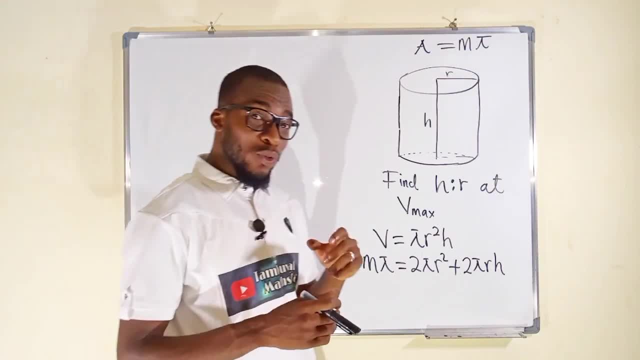 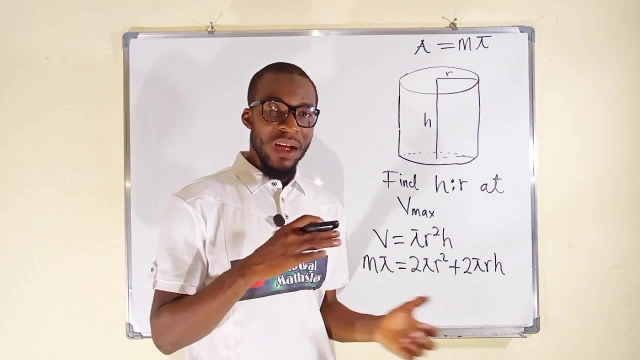 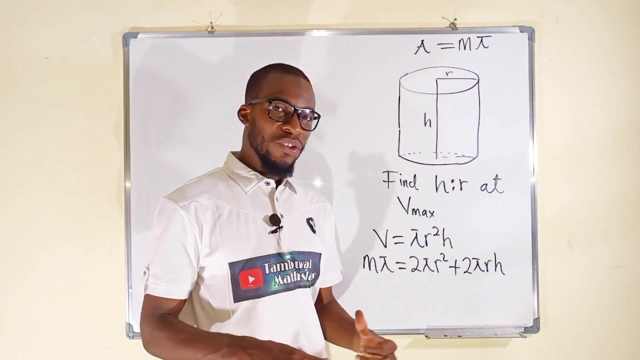 radius and the height. But I know subsequently, because we want to find the critical points, we have to differentiate v with respect to either r or h. So in this second equation we can make either r or h the subject, or get back into the first equation, differentiate and set everything to be equal to zero. 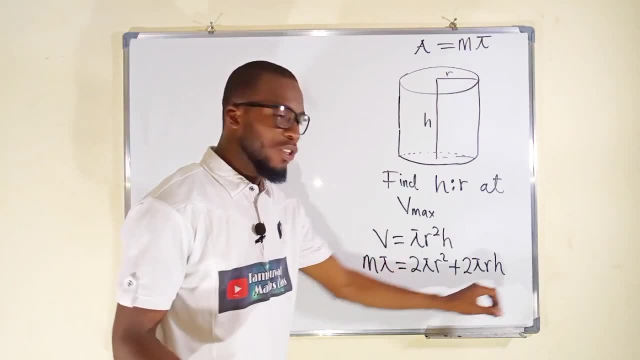 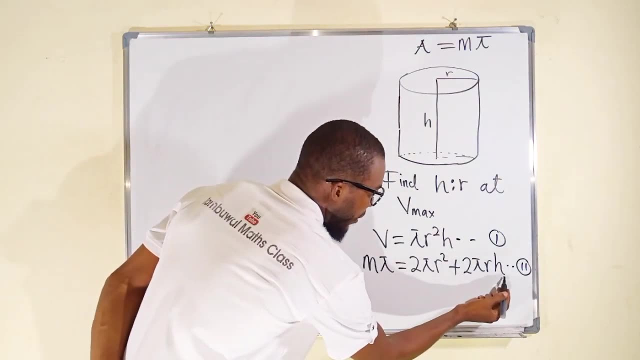 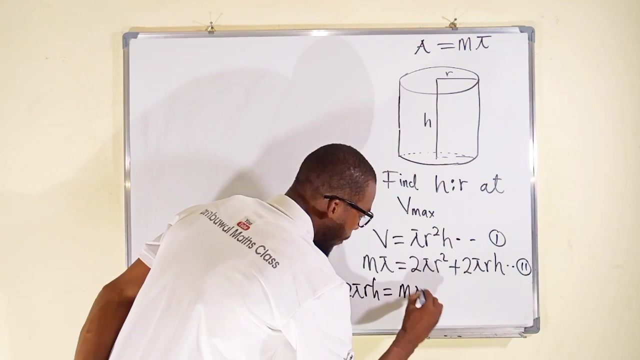 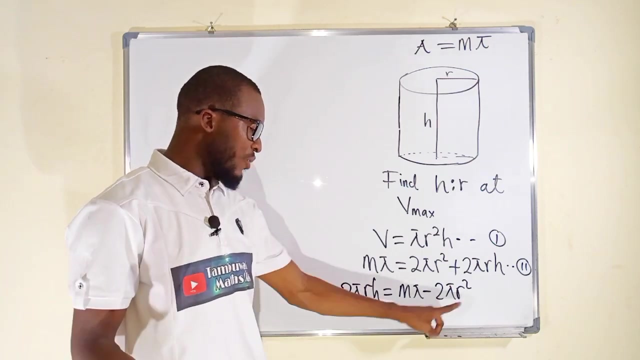 So for the second equation, we can make h the subject. So let me name this one, one, two. For the second equation, we can make h the subject: two pi r. h is now equal to m pi minus two pi r squared. Since we are looking for h, we can now divide each term. 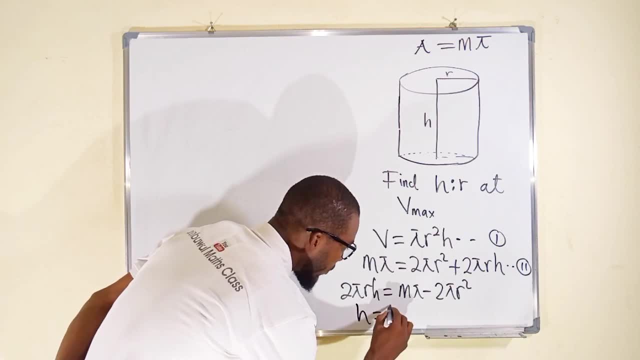 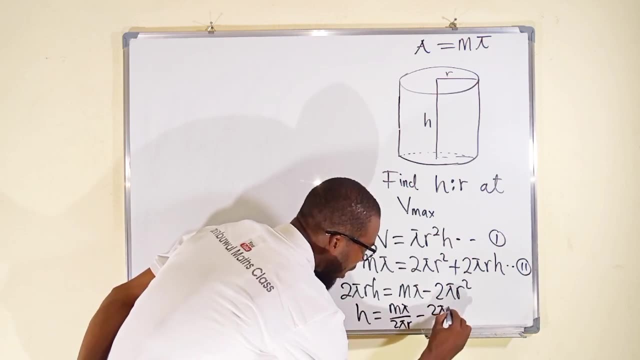 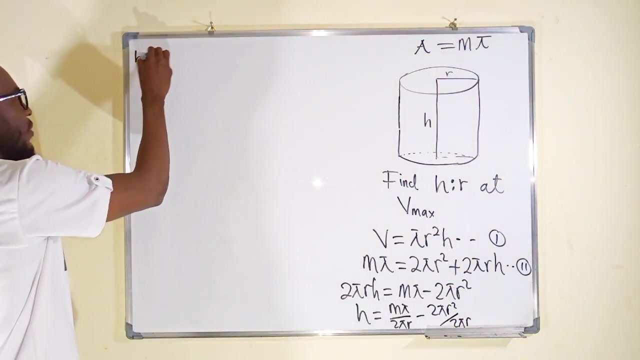 by two pi r and h is equal to m. pi over two pi r minus two pi r squared divided by two pi r. Let us simplify it. here We have: h equal to pi will cancel pi, leaving m over two r, The minus, The whole r. 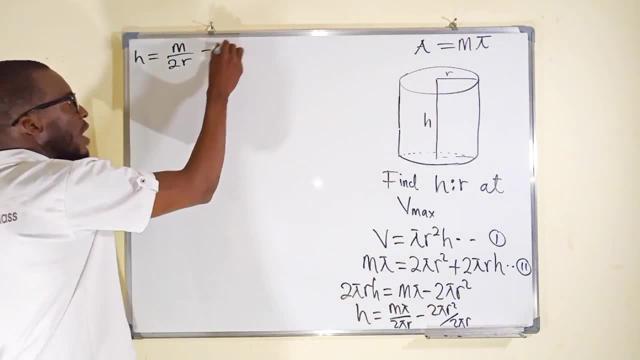 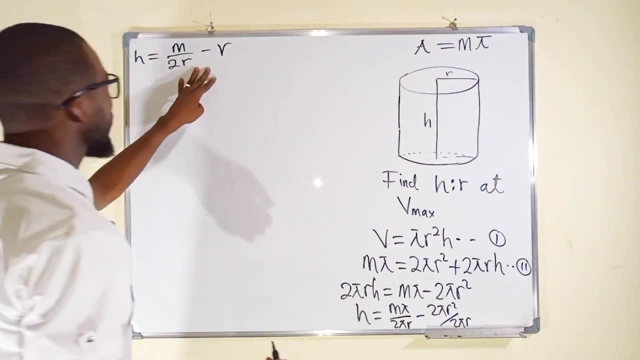 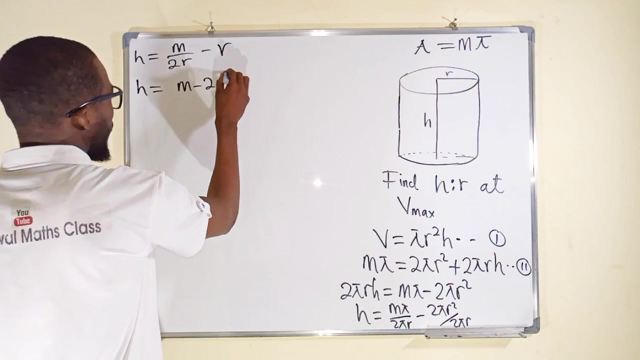 The whole r. All right, Okay. Okay, all of this will be equal to r, because 2 will cancel 2, pi will cancel pi. r squared divided by r is r. we can make this a single fraction: h equal to m minus 2. r squared over 2 r, remember. 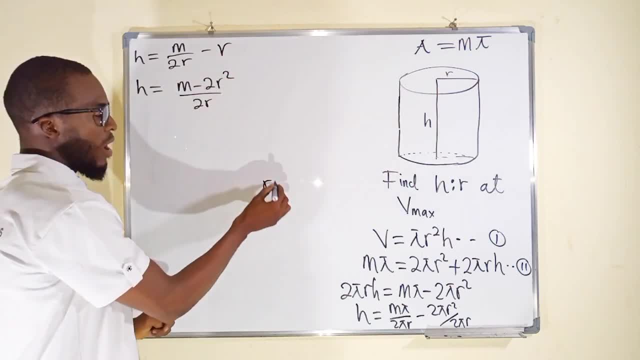 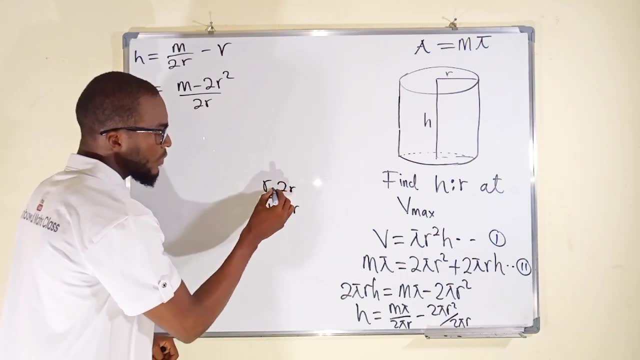 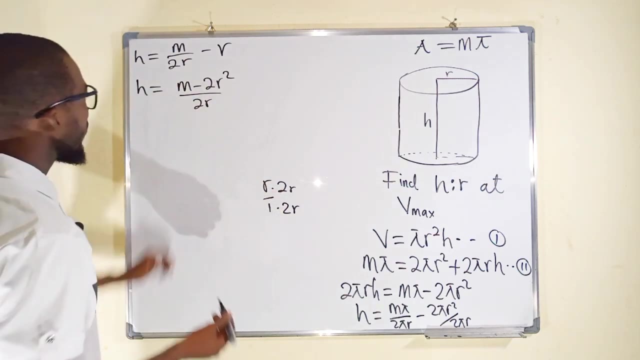 if you rationalize this, it is going to be r divided by 1 for common denominator. we can multiply the top and the bottom by 2 r. this is going to be 2 r squared m minus 2 r squared divided by 2 r. so you can see that h is equal to this, but from first equation we have h. so 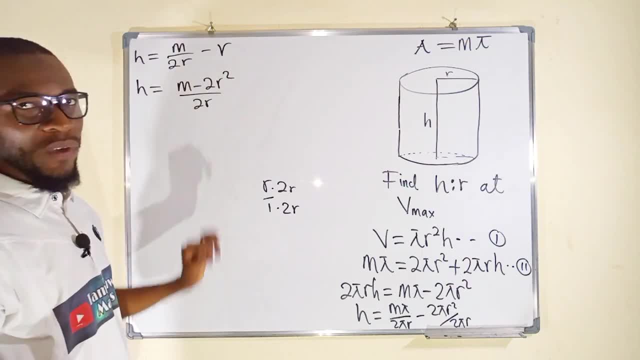 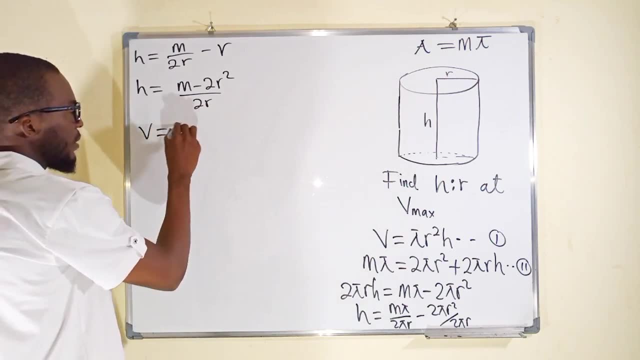 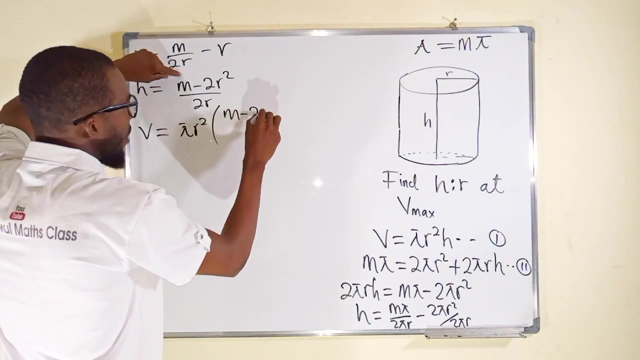 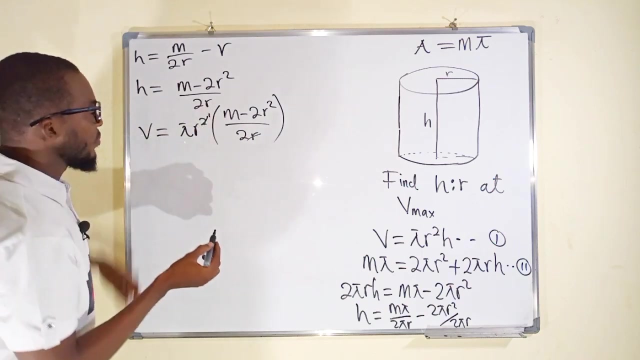 instead of h we can now substitute it with m minus 2 r squared over 2 r from that equation. so from equation one you can see, v will now be equal to pi r squared. instead of h we have m minus 2 r squared over 2 r. this single r will cancel one of the r's here, pi r multiplied by m. 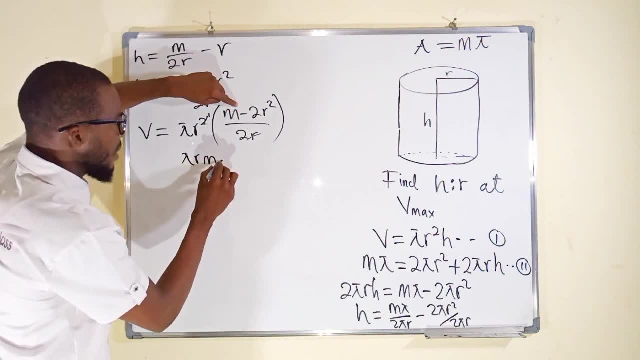 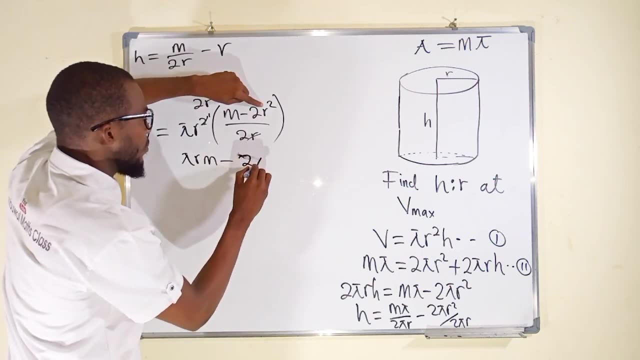 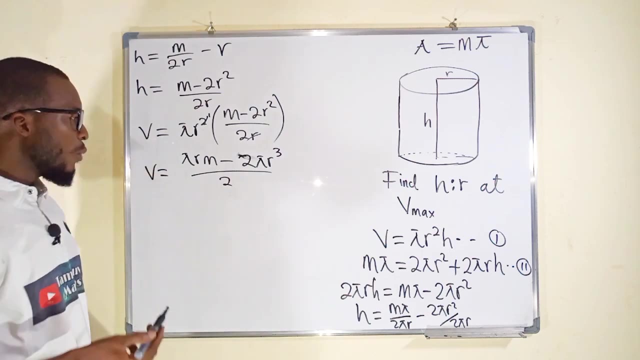 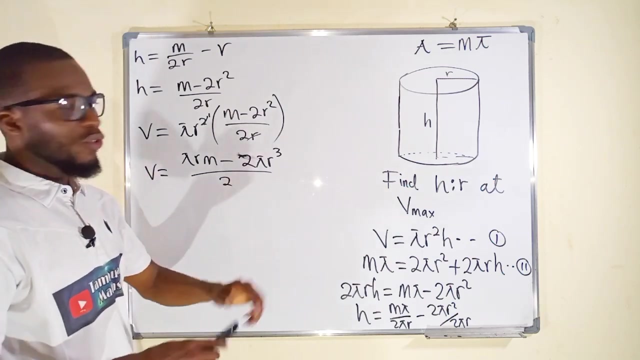 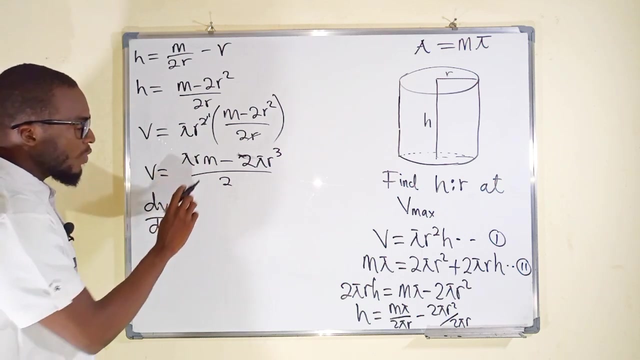 is pi r m. the minus pi r times 2 r squared is pi. okay, 2 pi r to the third power divided by 2, we have v here. so now let us find the critical points. by taking the first derivative of v with respect to r, we have dv over dr. remember m and pi here are constant if you differentiate. 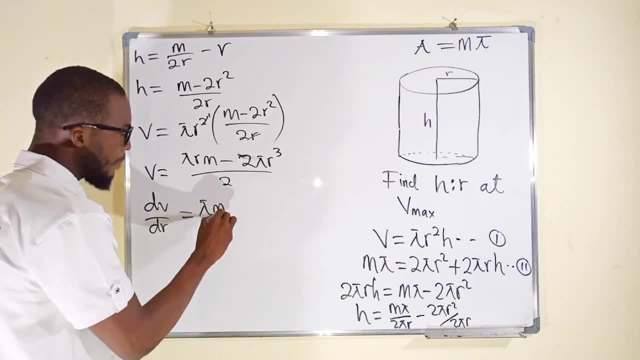 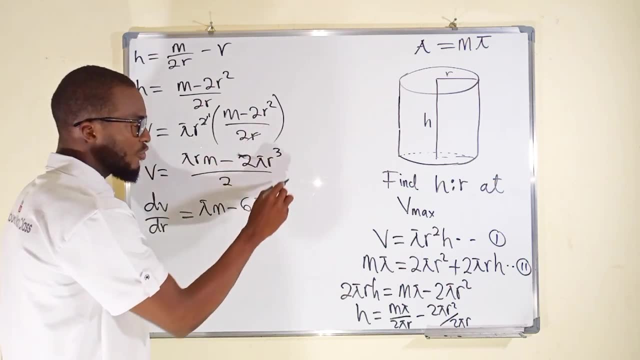 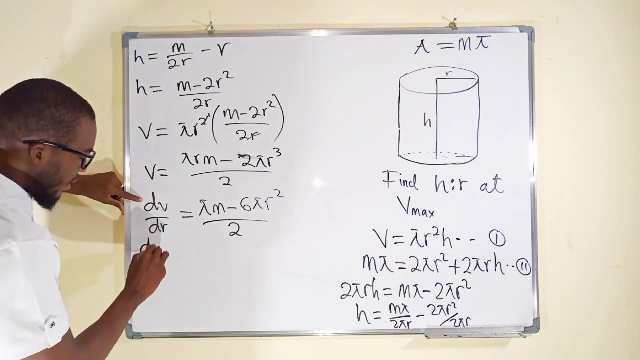 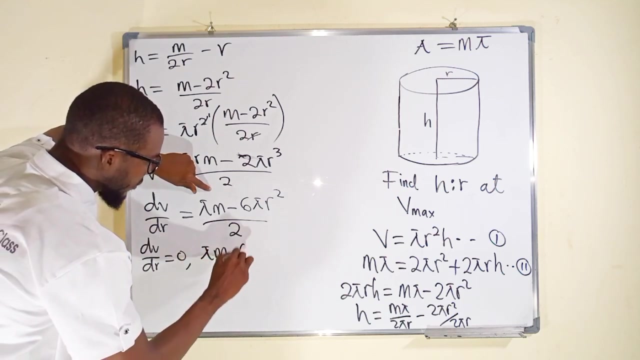 this you have pi m minus we have. 3 multiplied by 2 is 6 pi r to the 3 minus 1 is 2 divided by 2. so Now we want to set dv over dr to be equal to 0. And hence pi m minus 6 pi r, squared over 2, will be equal to 0.. 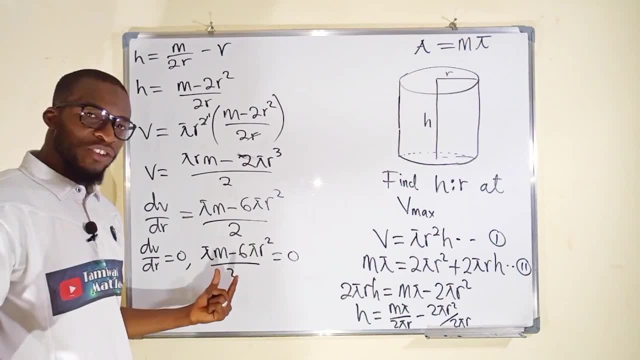 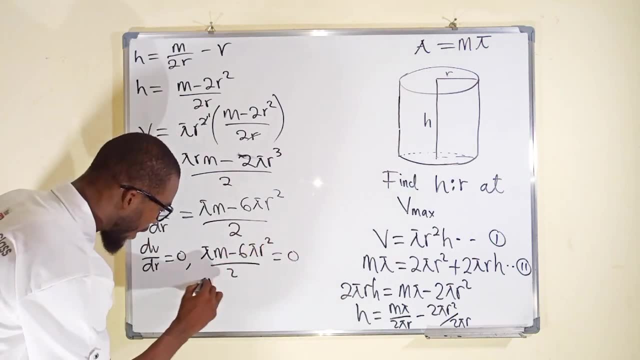 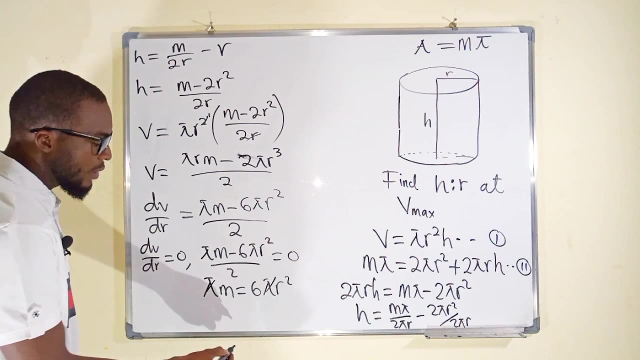 If you multiply both sides by 2, the fraction will be cleared up And you can take negative 6 pi r squared to the right and it becomes negative. We have pi m equal to 6 pi r squared. Pi will cancel pi. 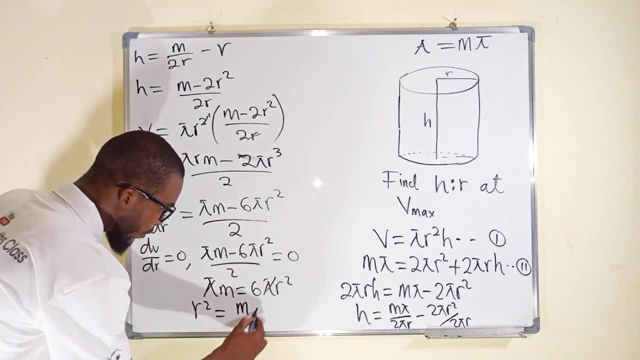 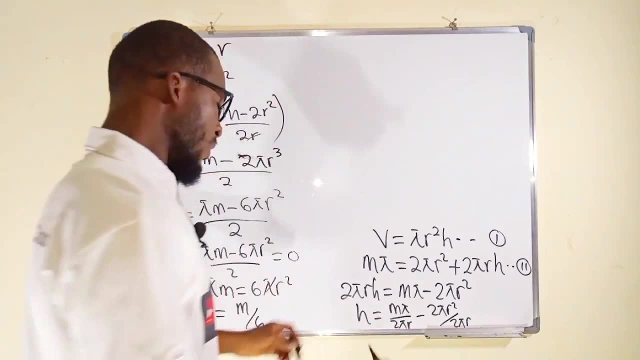 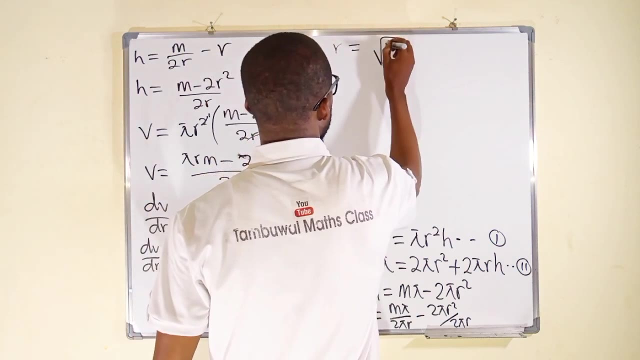 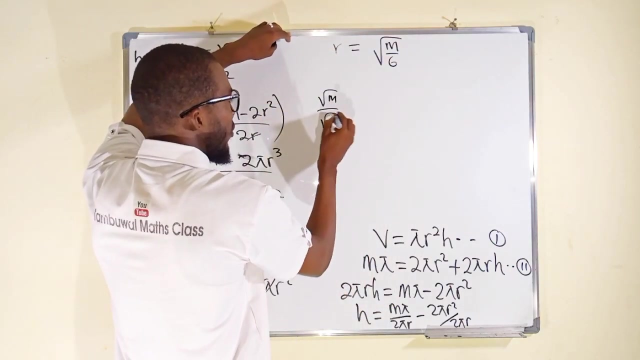 r squared will be equal to m over 6.. Now let us continue to the other side to find the value of r. r will be square root of m over 6.. So r is equal to square root of m over 6.. But remember, this can be written as square root of m divided by square root of 6, if you separate the roots. 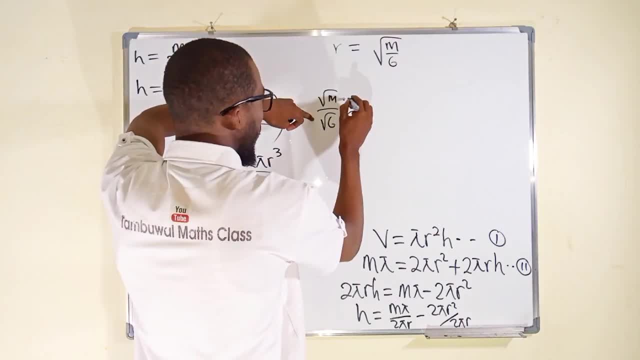 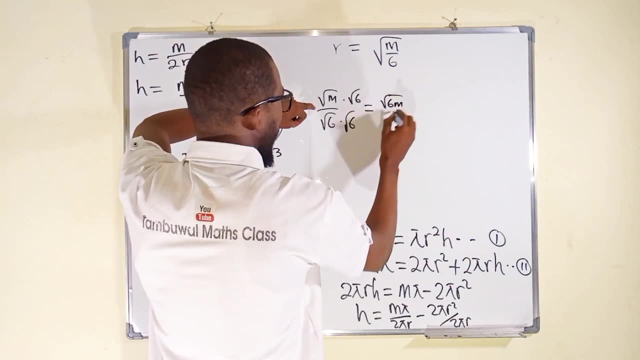 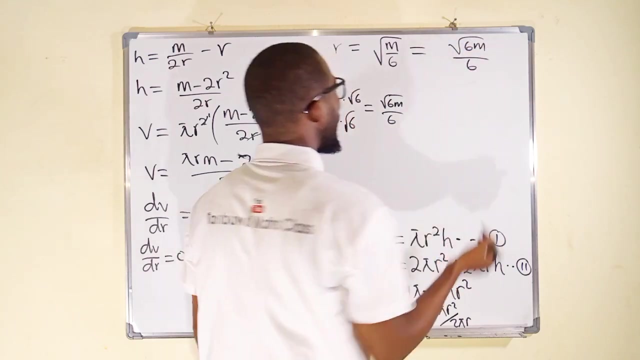 And you can multiply the bottom and the top by root 6 to rationalize the denominator, And this is equal to root of 6m divided by 6.. So this is equal to root of 6m divided by 6.. Now we have obtained the value of r, which is root of 6m over 6.. 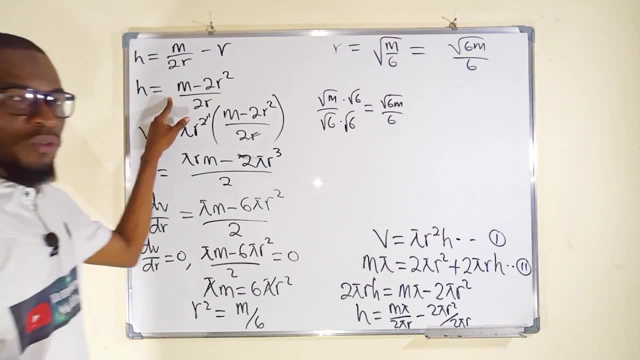 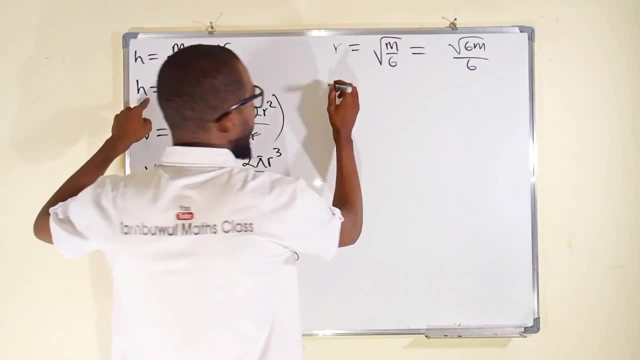 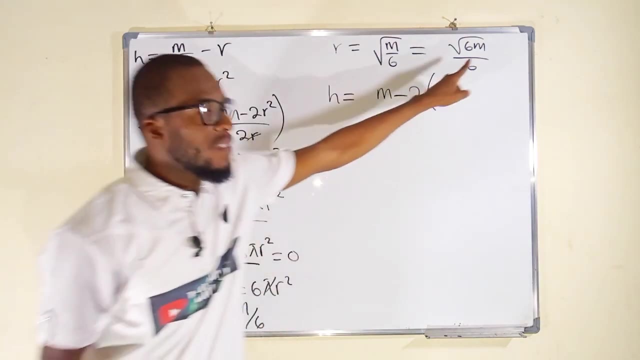 We can now subtract, We can now substitute it back into this equation to obtain the corresponding value of h. So h will be equal to m minus 2 multiplied by r. squared, This is r. If you square it. square will cancel square root to the top. 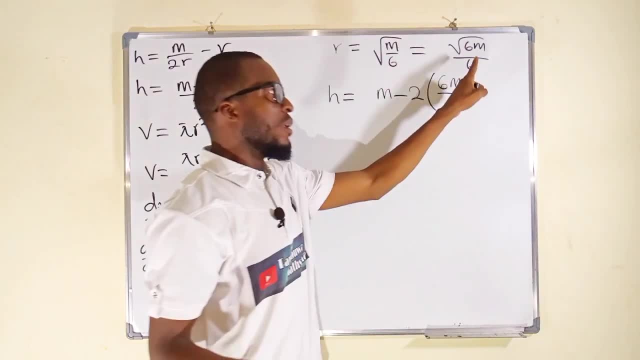 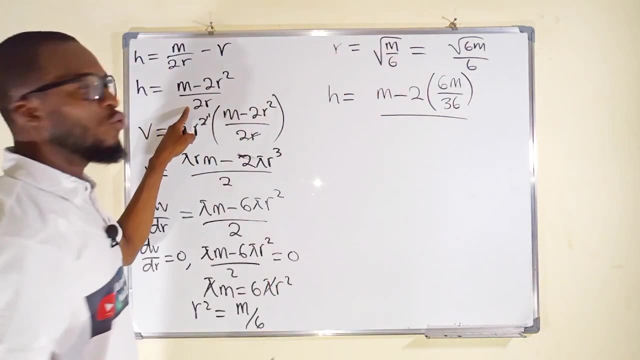 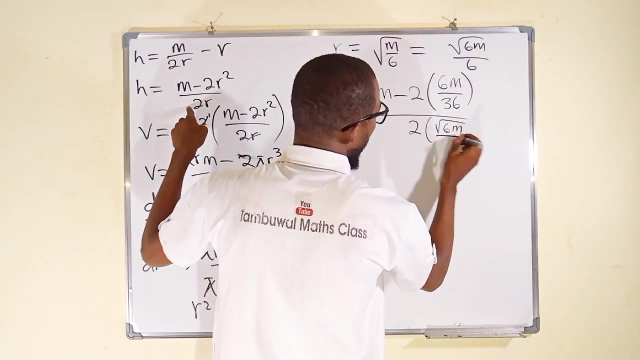 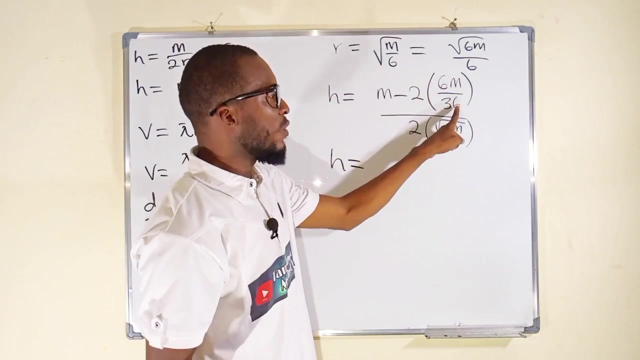 We have 6m. Divide by Square the bottom, You get 36.. Denominator is 2r, which is 2 multiplied by the r is root of 6m over 6.. Let us further simplify: h is equal to 6 can go into 36 6 times and 2 can go into that 6 3 times. 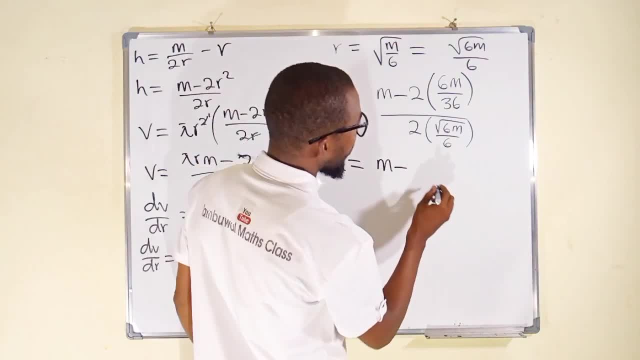 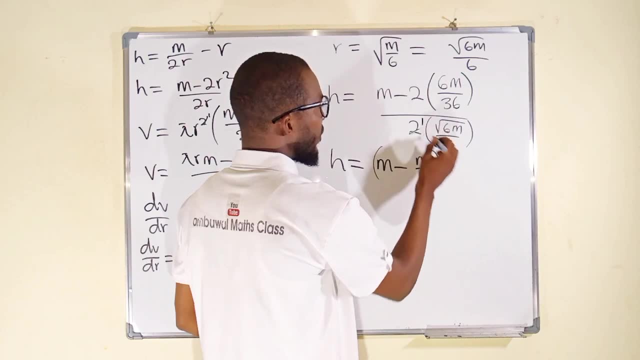 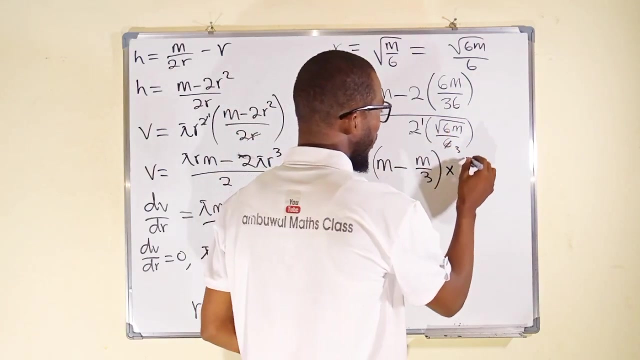 So this will be m minus m over 3.. 2 can go into 2 one time and 2 can go into 6 three times. But we can now multiply and take the reciprocal of this. Multiply by 3 over root of 6m. 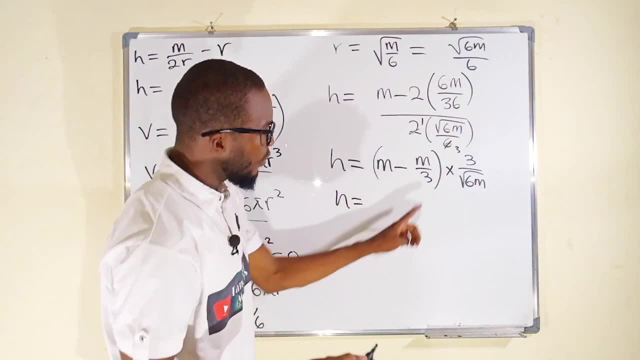 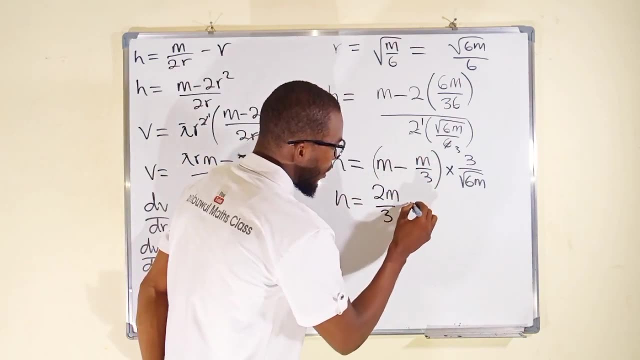 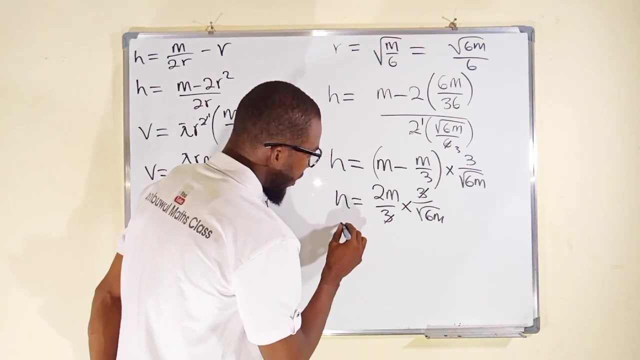 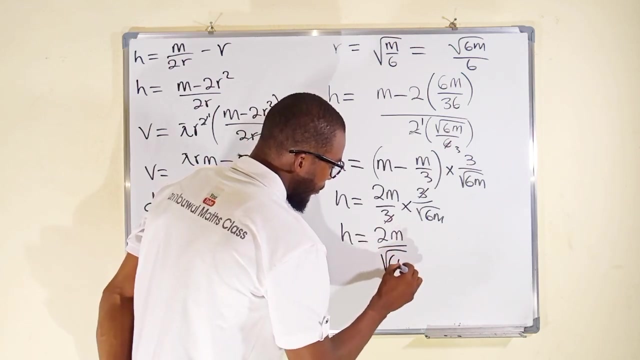 h is now equal to 3. multiplied by m is 3m minus m is 2m over 3.. If you multiply with 3 over root of 6m, 3s will cancel. Finally you can see we have h to be equal to 2m over root of 6m.